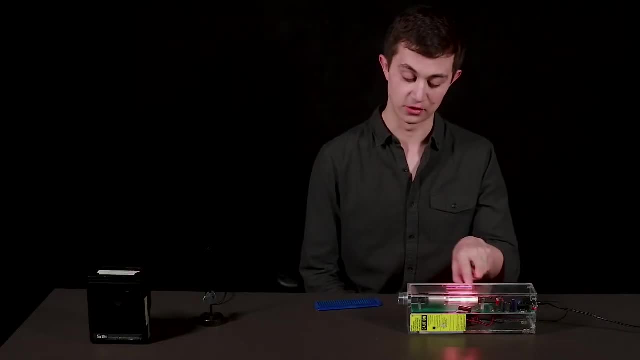 cavity. This is the light bulb. This is the laser beam. This is the laser beam. This is the laser beam. This is the body of the laser. and as they're doing that, as they go through the gain medium, the photons become coherent with one another so that they go back and forth together, and this makes it so that 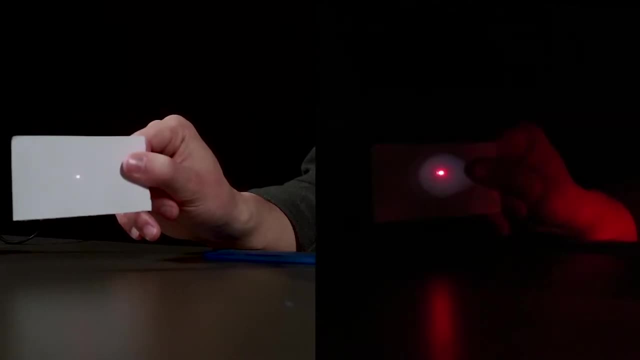 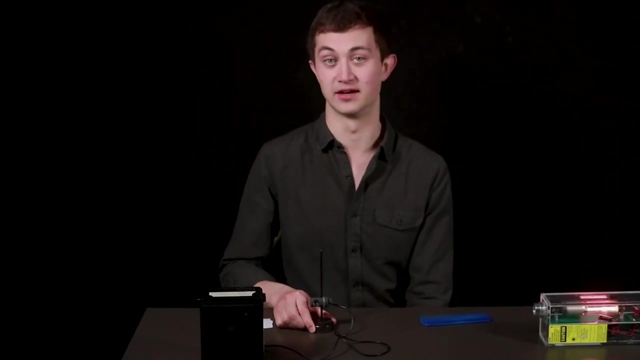 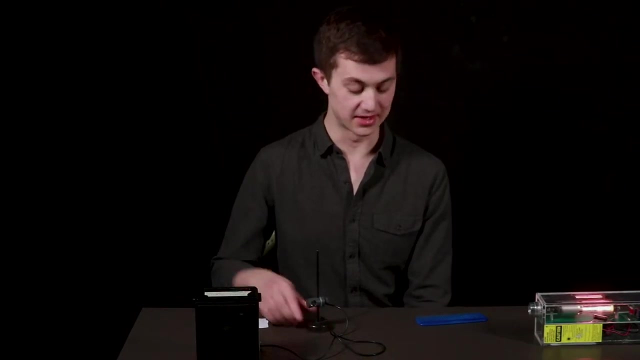 the output of the laser is highly directional, single color and coherent. Now let's talk about the detector. Over here we have a silicon detector which turns light signal into electrical signal, and we can do all sorts of different things with this, but in this case we'll take the beam coming. 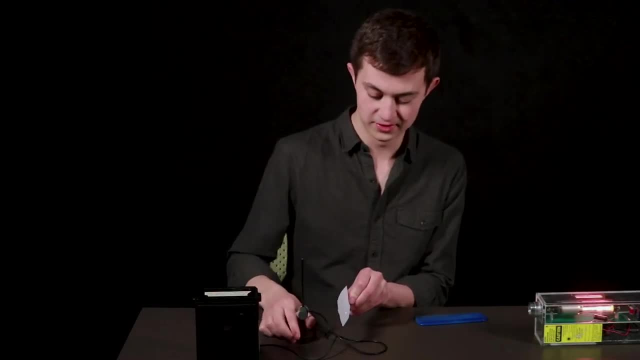 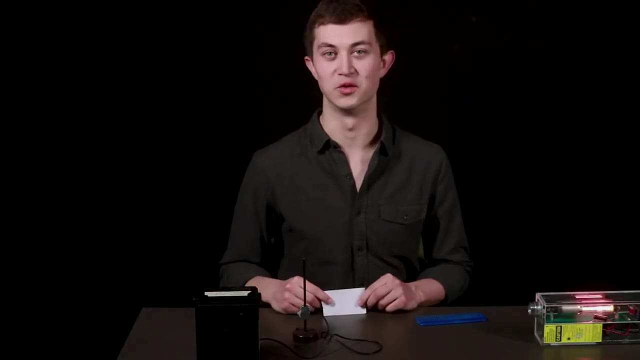 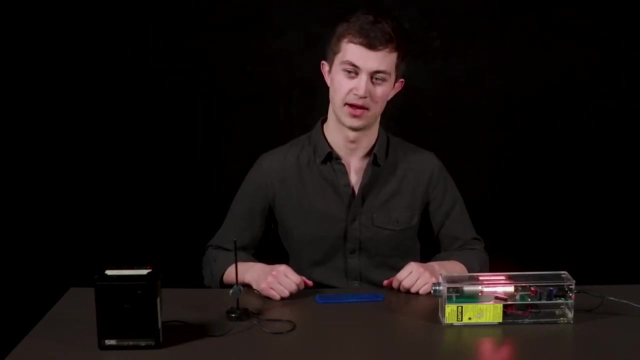 out of our laser And we'll align our detector with the laser beam and run it into a speaker and we'll see what sorts of fun things we can do with that. Finally, let's talk about the demo. First question we ask ourselves is: can we make sound by blocking light? That's an interesting question, So we can take an ordinary. 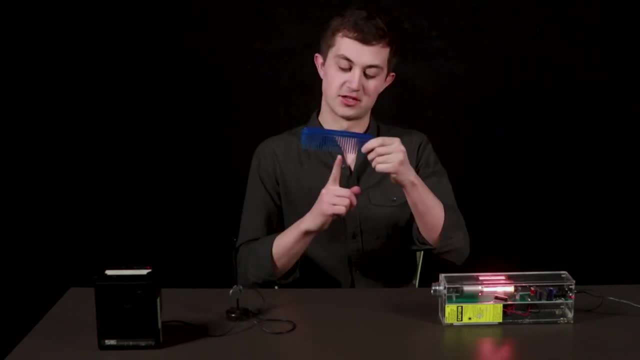 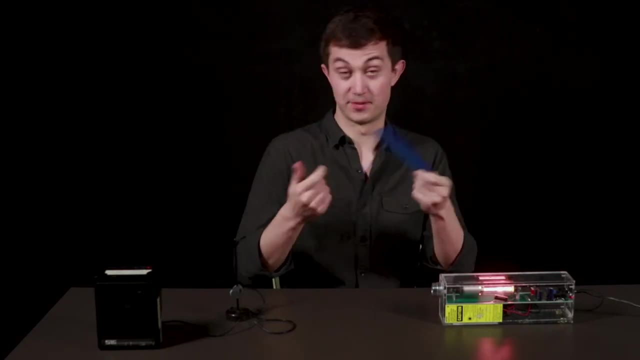 comb and do this. When I run the comb across my fingers, the comb will tend to bump my fingers up and down as I move along, As you might be familiar with, But as I run the comb in front of my eye, it also does the same thing with. 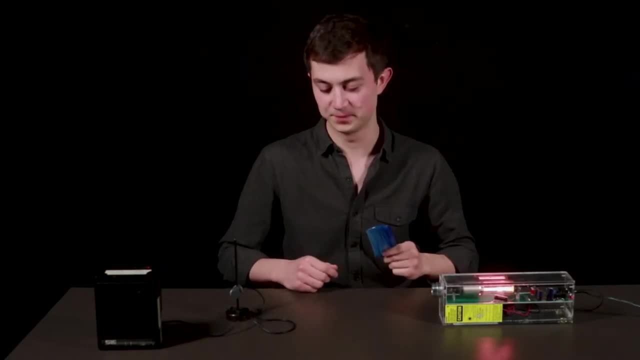 the light. So if I put it in front of the laser it's also going to modulate the light up and down, up and down, up and down. And by changing the speed at which I move the comb through the laser I can generate a. 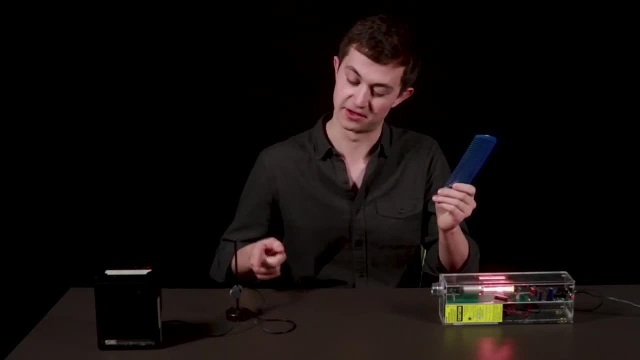 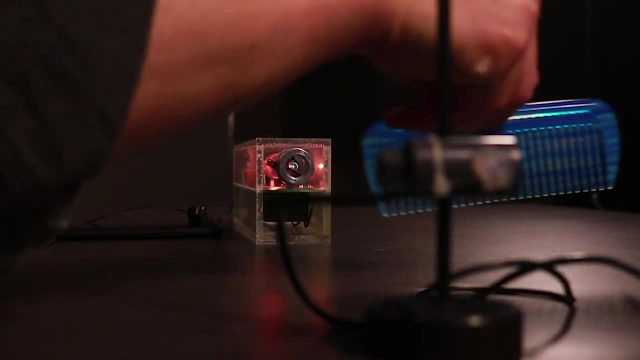 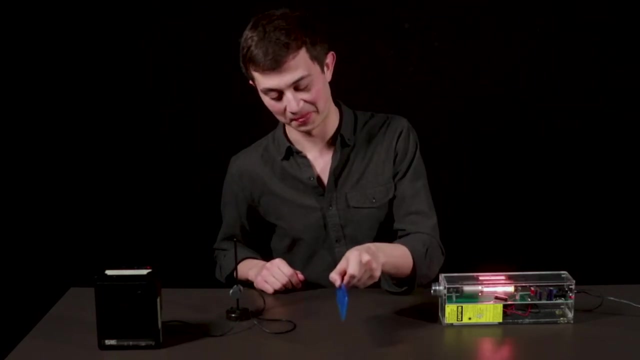 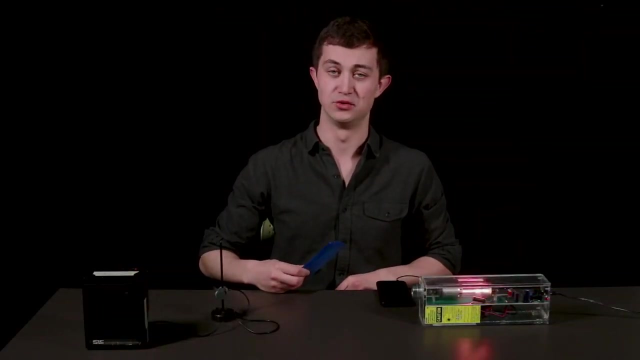 frequency this way that my ears can interpret, because I have my detector hooked up to a speaker. So let's try it out. So if I go slowly, You're barely audible. If I go quickly Becomes more of a sound- Pretty fun. So now that we've seen one way that we can turn blocking light into generating sound, is there? 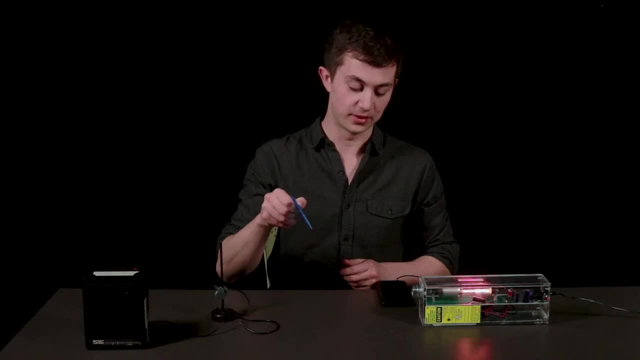 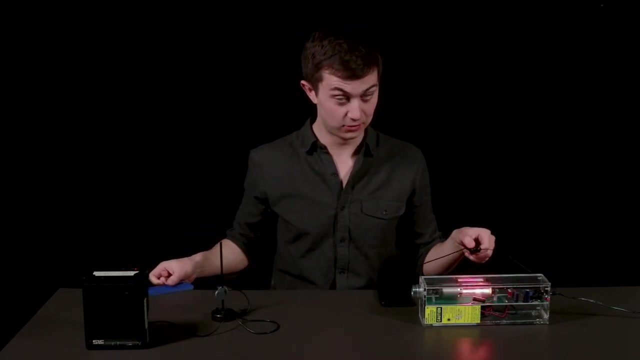 another way that we can do that. So we just put the comb into the laser beam and we selectively blocked, turned on and off the laser beam as it appeared on the detector over here. Instead of doing that, we can turn the laser on and off directly by running a cable into it and connecting a device that can.